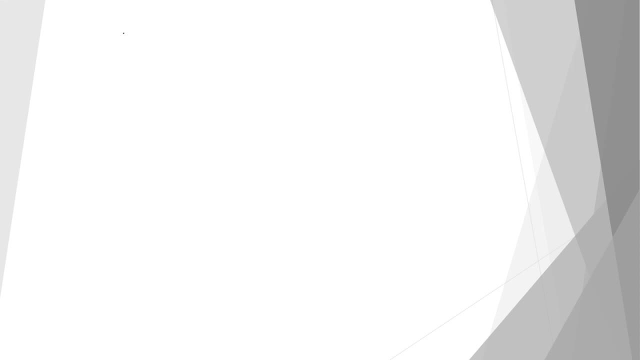 the number by which we can divide the number. So first of all we will see the divisors of 6.. You know, every number is divisible by 1 and the number itself Means if you multiply this 1 into 6, you will get 6.. Now, second number: 6 is a even number, So you can divide 6 by 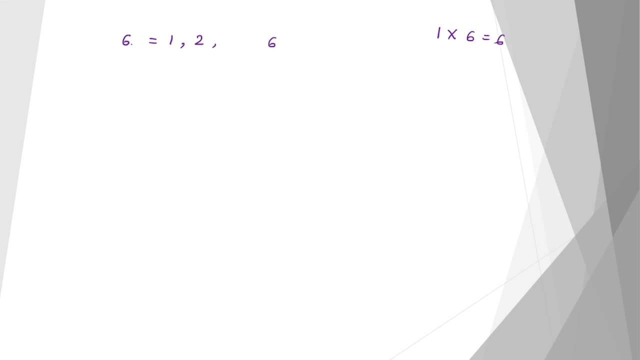 2 and after dividing 6 by 2 will get 3.. Means, if you multiply 2 into 3, you will get 6.. So 1.. 2, 3 and 6.. These are all divisors of 6.. Let us take one more sum. The bigger number will. 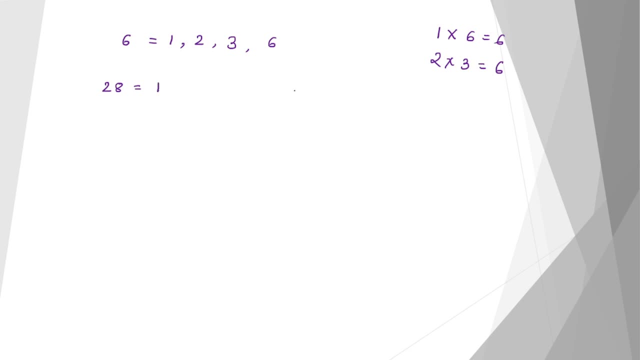 take 28.. Again, you know the number is divisible by 1 and the number itself. So we will write like this: Then 28 is even number, It is divisible by 2.. When you divide this 28 by 2, you will. 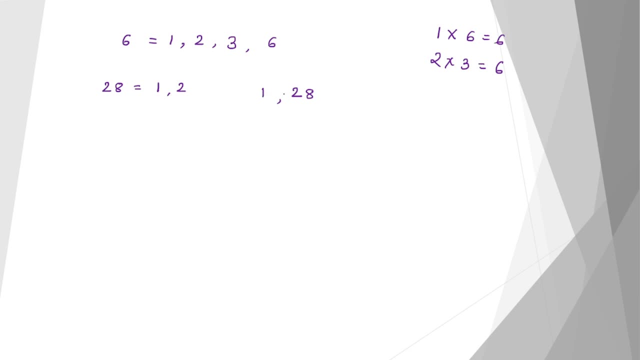 get 2, ones are 2 and 2, fours are 8.. Then check for 3, 8 plus 2 plus 8, 10.. So 10 is not divisible by 3. So this number is not divisible by 3. Unit place is 8.. So this: 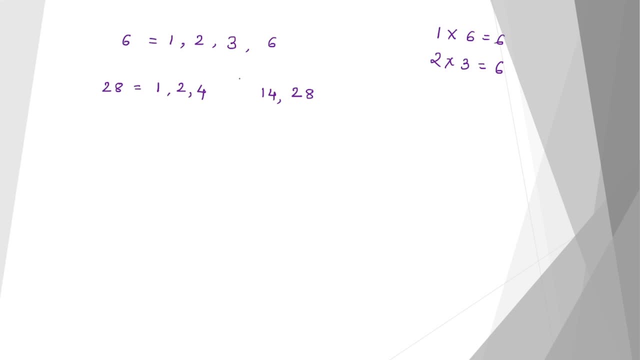 number is divisible by 4.. So 4, 7s are 28.. So these are all divisible by 8.. So this the multiples, sorry, these are all the divisors of 28 if you check the pairs 1. 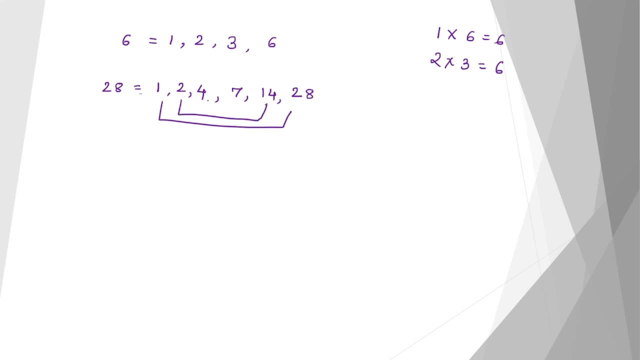 into 28, 28, 2 into 14, 28, 4 into 7. 28 means these are all divisors of 28. now, these are the small numbers. you can write like this directly, but if you get bigger number then you don't know how much place you have to keep in between. 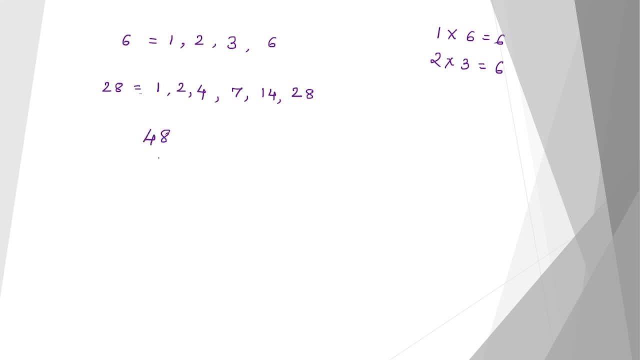 and all. so we can write like this, draw a line like this: if you divide 48 by 1, you will get 48, then 48 is a even number. check for 2: 2, 2s are 4, 2, 4s are 8, then 8. 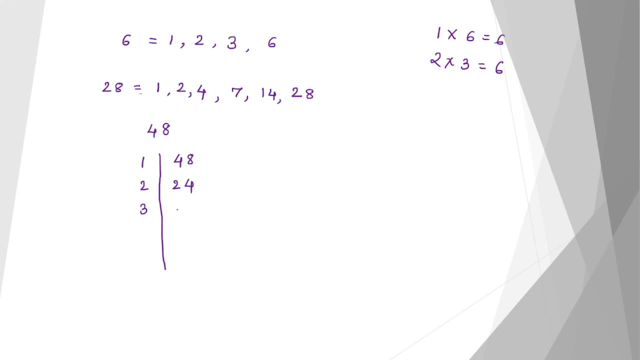 plus 4, 12, so you can divide it by 3. so 3, 1s are 3, 3, 6s are 18. unit place is 8. it is divisible by 4. 4 ones are 44. twos are 8. this number is divisible by both 2 and 3, so it is. 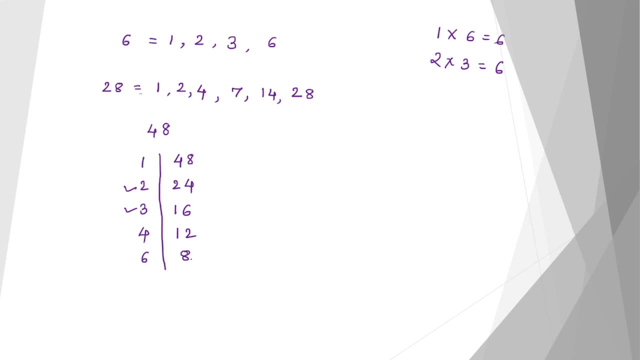 obviously, divisible by 6, 6, 8s are 48. you cannot divide it further by 7, 8, 9. so these are the all fact, all divisors of 48. so the divisors of 48. you can write it as 1, 2, 3, 4, 6. 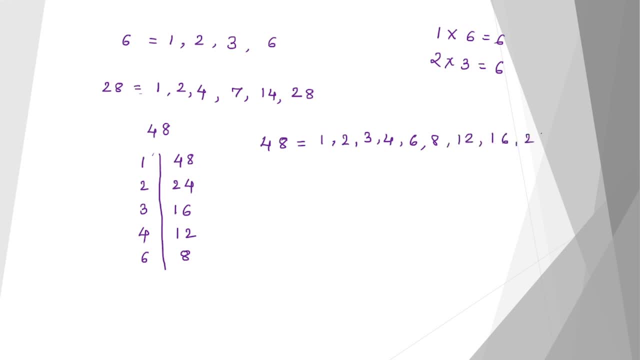 12, 16, 24 and 48. these are all divisors of 48. let us go for another number, that is 72, because it is a bigger number. just draw a line like this: 17, then you know it is divisible by 2 because it is a even number. 2, 3 is a, 6, 2, 6 a 12. what we? 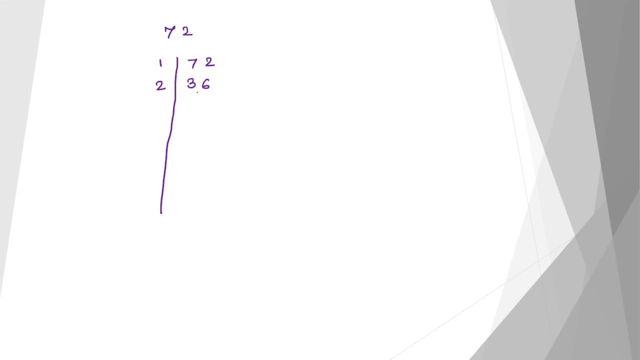 are doing? we are just dividing this number by 2 and whatever quotient you are getting, you are writing here. so next number is 3, 3, 2 is a 6. 3, 4 is a 12. then it is divisible by 4. also 4. 1 is a 4, 4, 8 is a 32. 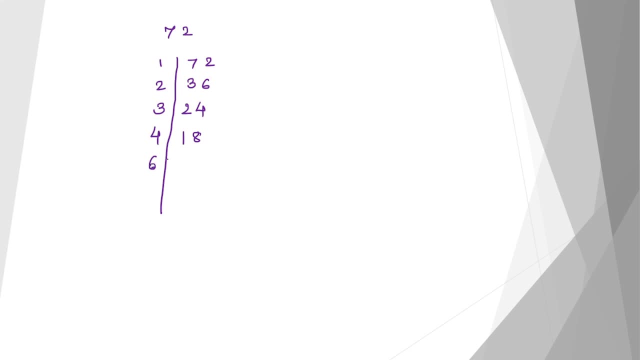 if it is divisible by 2 and 3, this number is also divisible by 6. 6 ones are 6, 6, twos are 12. then this number is divisible by 8 also. so 8, 9s are 72. you get nearby number. so this is the end of the sum. so you can write the divisors of. 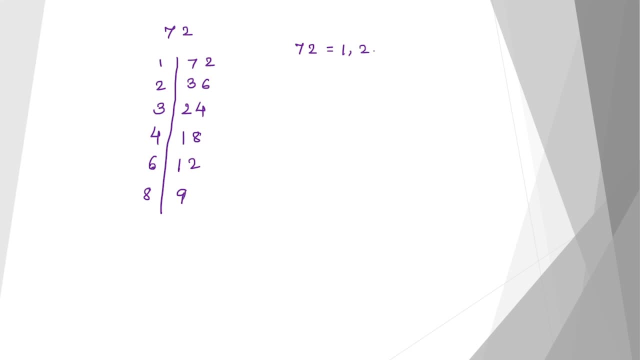 72 is equals to 1, 2, 3, 4. so you can write the divisors of: 72 is equals to 1, 2, 3, 4, 6, 8, 9, 12, 18, 24, 36 and 72. these are all divisors. you can write here divisors of. 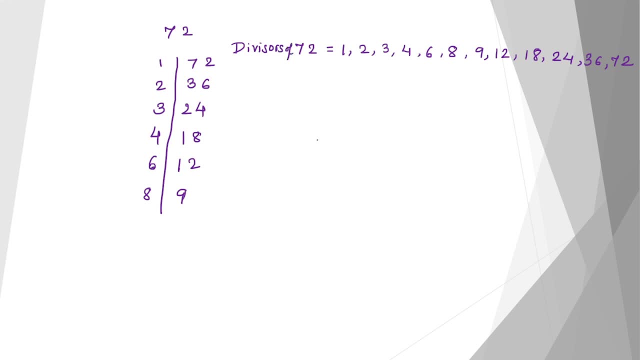 72. like this you can write: let us take one more sum: 63, so like this: 1 and 63. you know, this number is divisible by 3, so 3, twos are 6, 3 ones are 3, then 7, 9s are 63. 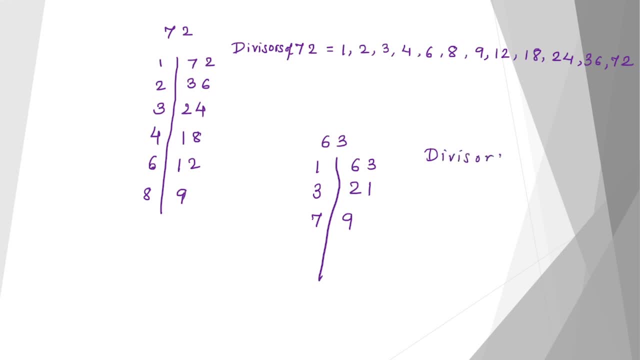 so the divisors of 63 is equals to 1, 3, 7, 9, 21 and 60. so this way we can find the divisors of 60. so this way we can find the divisors of 60. so this way we can find. 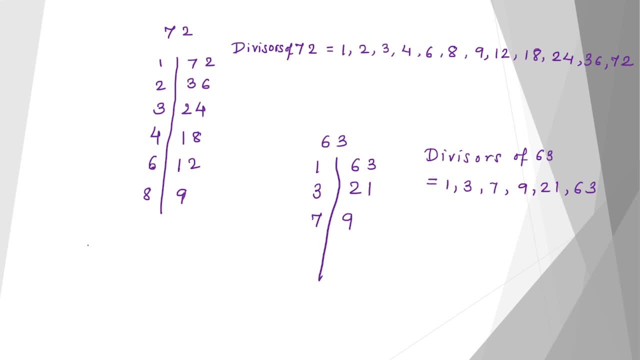 the divisors of any number. Now I will give you one sum to solve. Your question is: find divisors of number 42.. Your answer you can write in the chat box. If you like this video, don't forget to subscribe the channel and share it with your friends. Thank you.